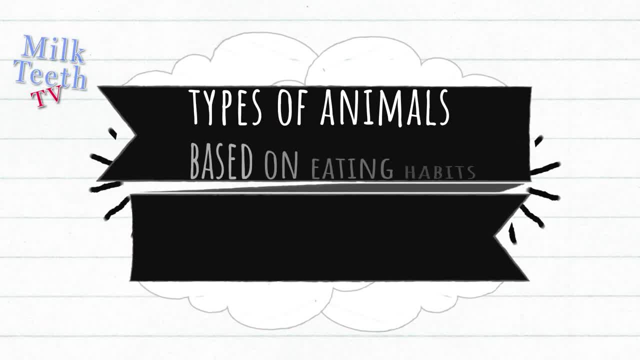 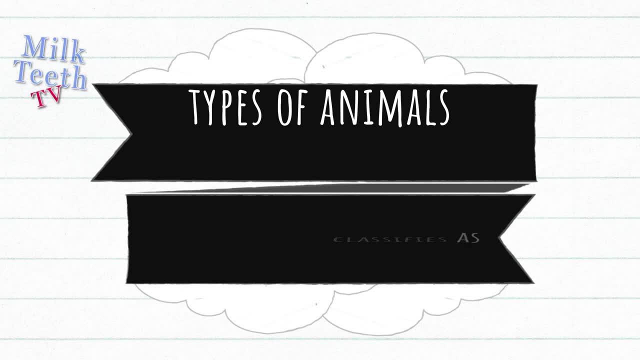 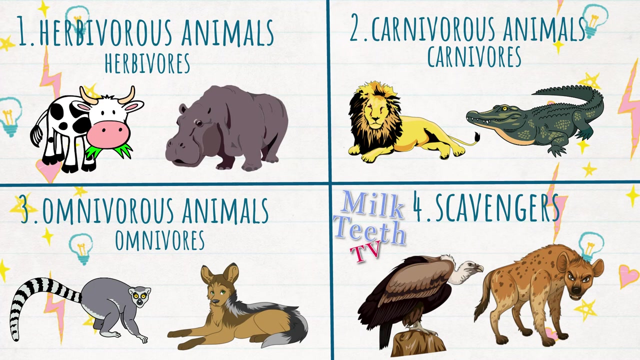 Types of Animals. Based on eating habits. animals are classified as herbivorous animals, carnivorous animals, omnivorous animals and scavengers. Herbivorous animals are also called herbivores, Carnivorous animals are called carnivores, Omnivorous animals are called omnivores and scavengers are called scavengers. 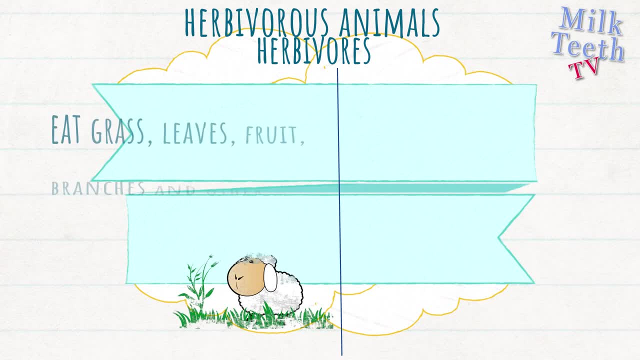 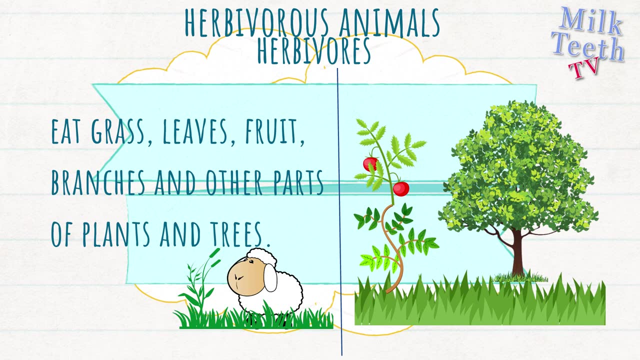 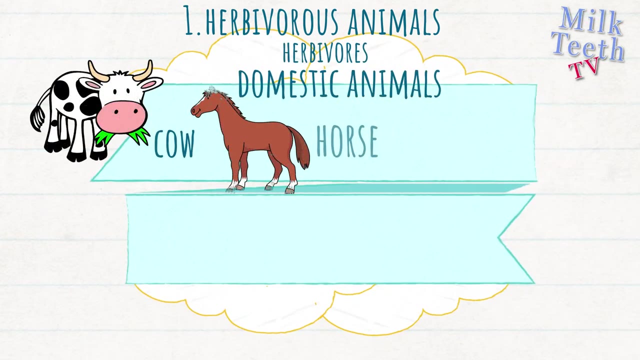 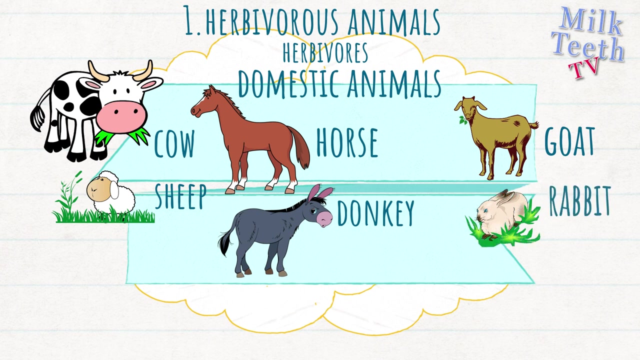 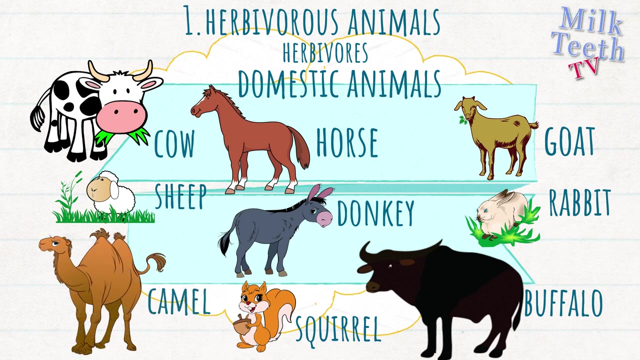 Herbivorous animals are the herbivores. These eat grass, leaves, fruits, branches and other parts of plants and trees. Domestic animals like cow, horse, goat, sheep, donkey, rabbit, squirrel, buffalo and camel are all herbivorous animals, ie they depend on plants and trees for their food source. 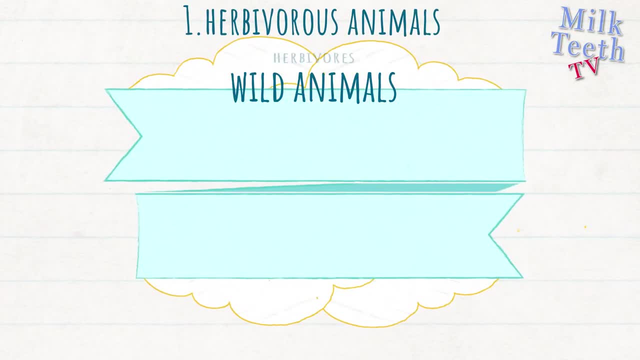 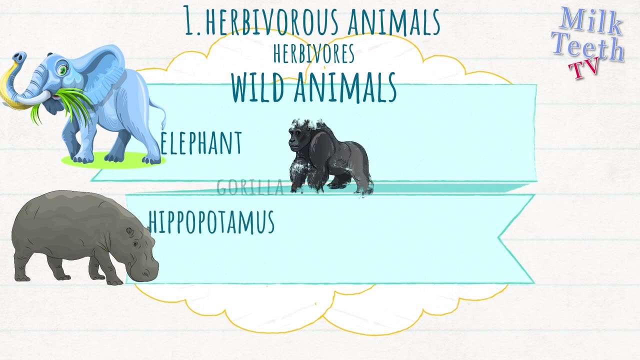 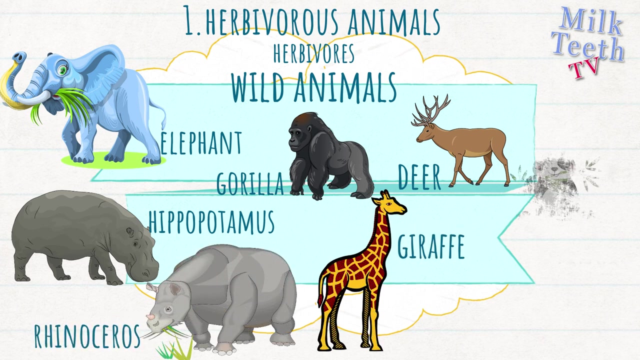 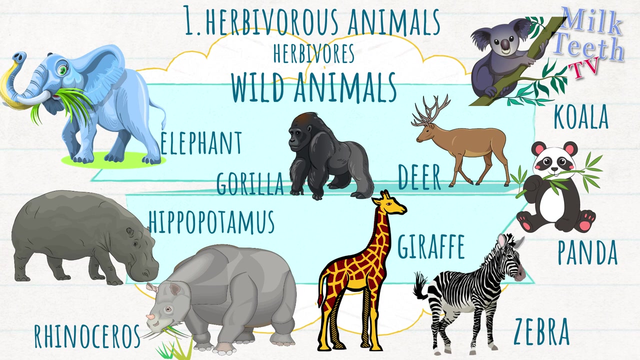 Many wild animals like the elephant, hippopotamus, gorilla, deer, giraffe, rhinoceros, panda, koala and zebra are also herbivorous animals or herbivores. These also depend on plants and trees for their food source. 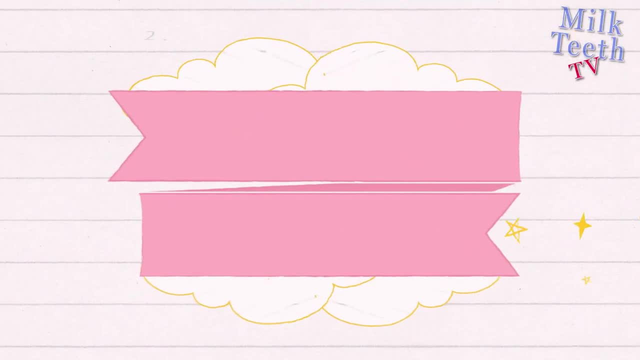 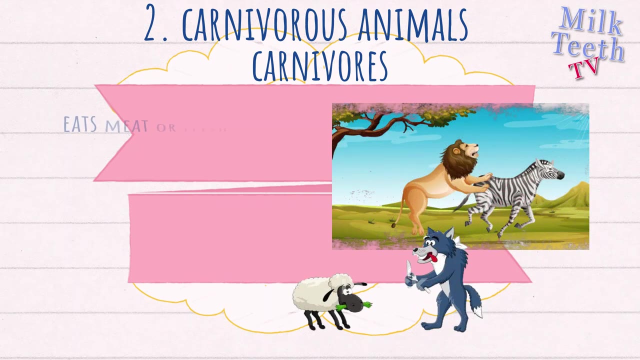 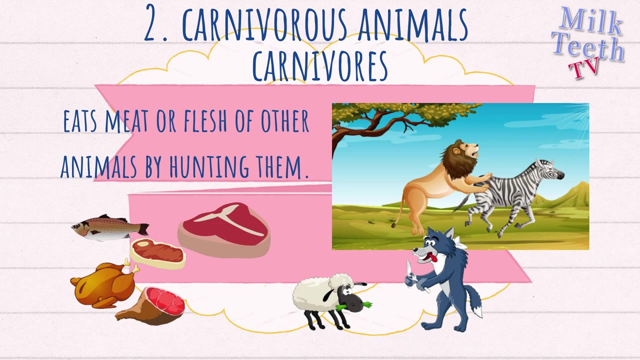 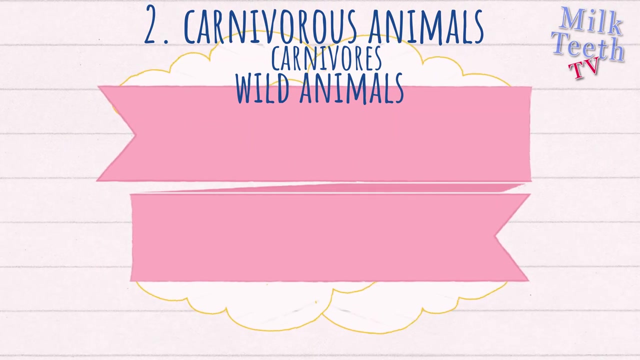 Carnivorous Animals are also called carnivores. These animals eat meat or flesh of other animals by hunting them. Please note that these are called carnivorous animals or simply carnivores. Mostly the wild animals are called carnivores And the wild animals are the carnivorous animals. 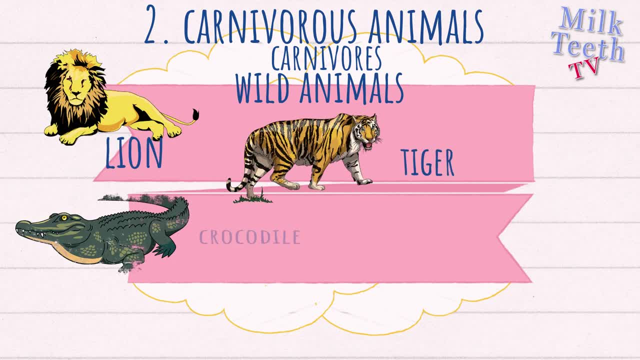 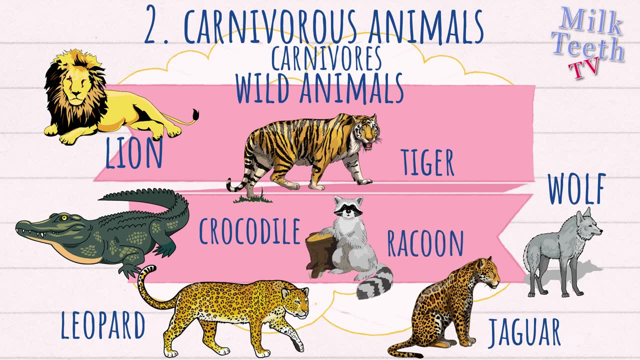 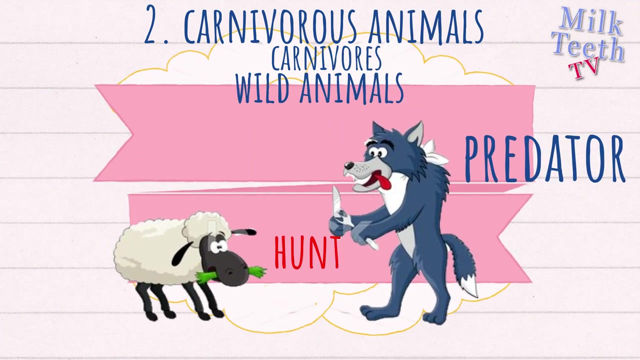 Animals like Lion, Tiger, Crocodile, Wolf, Leopard, Jaguar, Raccoon and Hyena are the carnivorous animals or the carnivores. The carnivores are also called predators because they hunt or kill the animals that they want to eat. 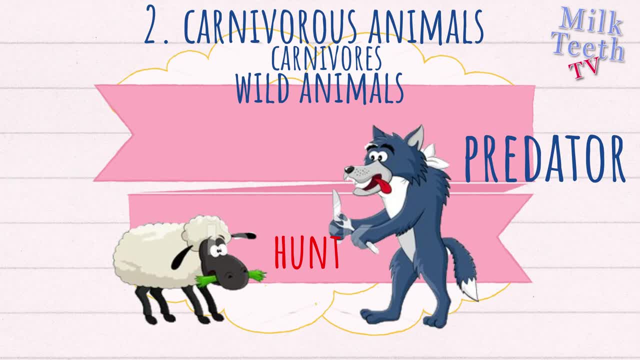 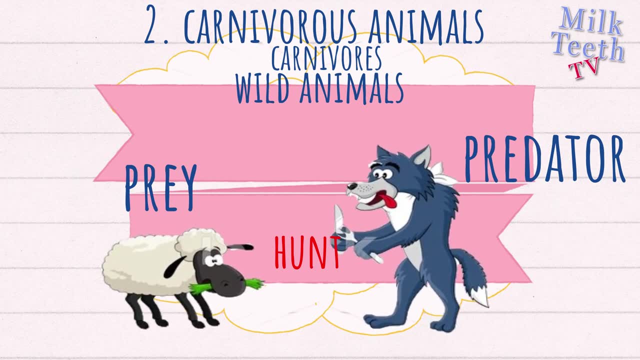 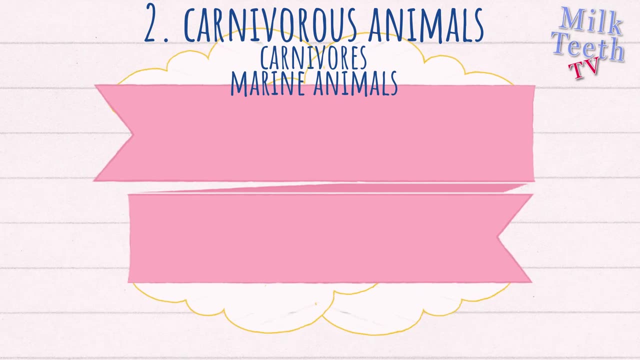 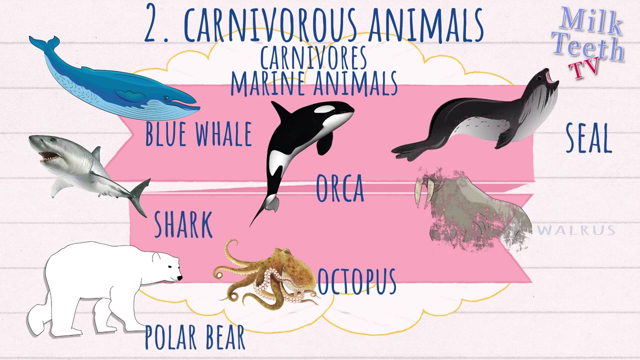 The animals which these predators hunt down are called their prey. They eat the flesh of the prey as their food. Many marine animals are also carnivorous animals or carnivores: Animals like the Blue Whale, Orca, Octopus, Shark, Polar Bear, Seal, Walrus and Sea Otter. 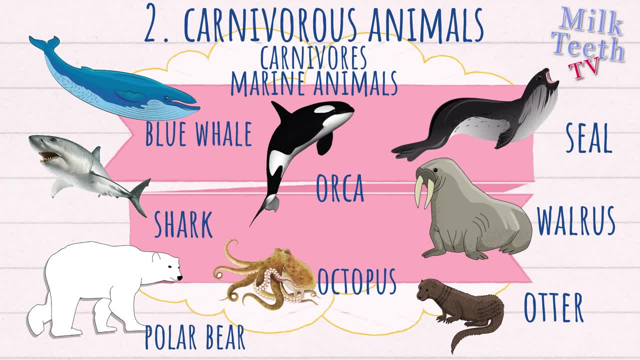 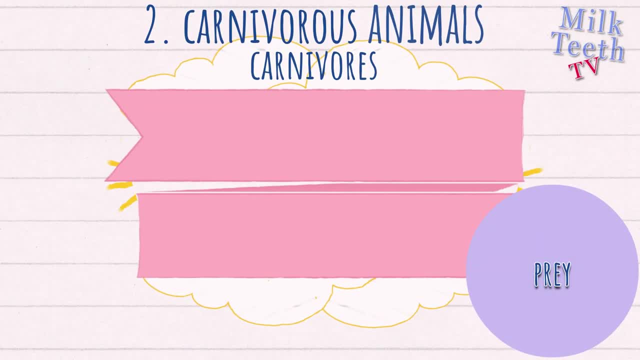 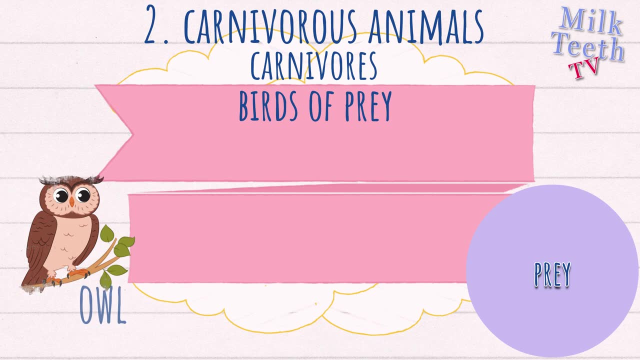 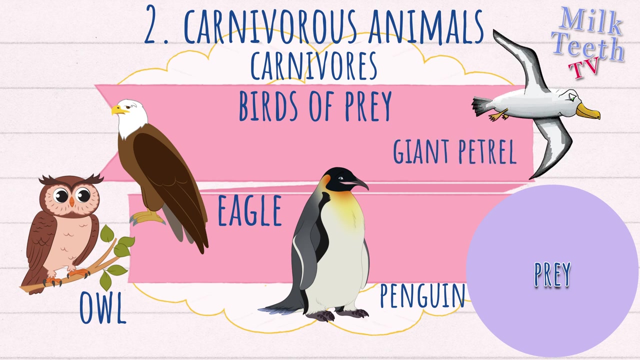 are all carnivorous animals. These hunt on fish and other sea animals for their food. Many birds are also carnivorous in nature. These are called birds of prey. Birds of prey are also carnivorous in nature. Birds like Owl, Eagle, Penguin and Giant Petrel are all carnivorous birds or carnivores. 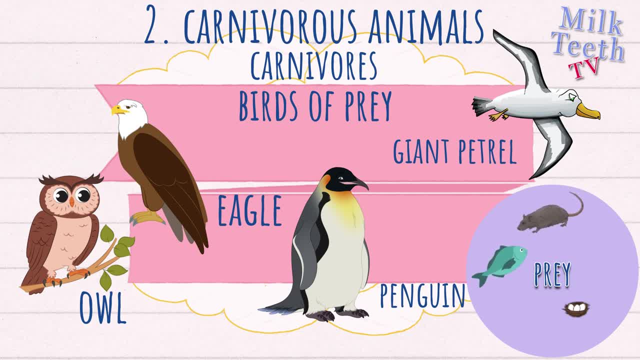 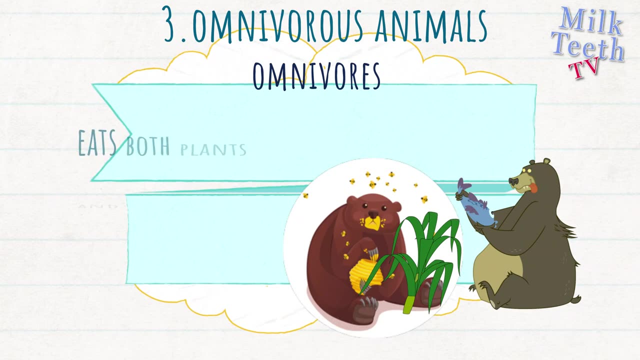 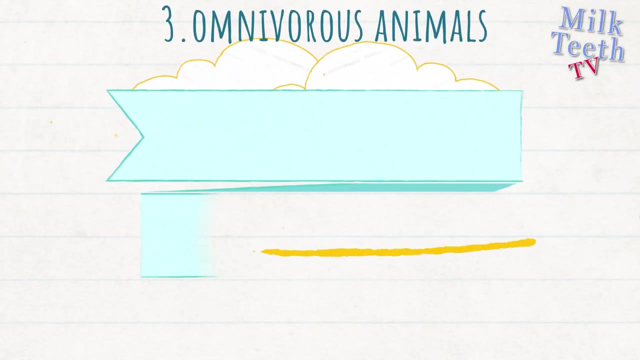 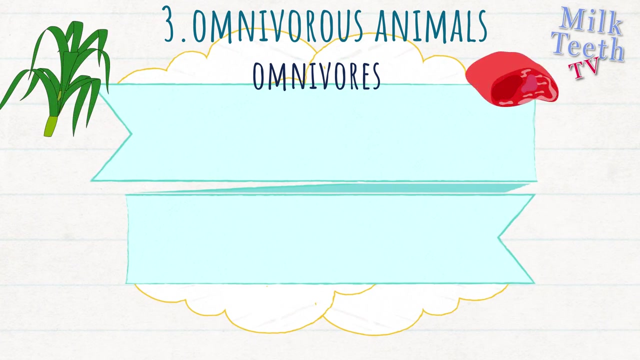 These hunt on other small animals, eggs of other birds, insects and other organisms for their food. Omnivorous animals are the omnivores. These eat both plants and meat of animals. Several animals and mammals eat both plants as well as flesh of other animals. 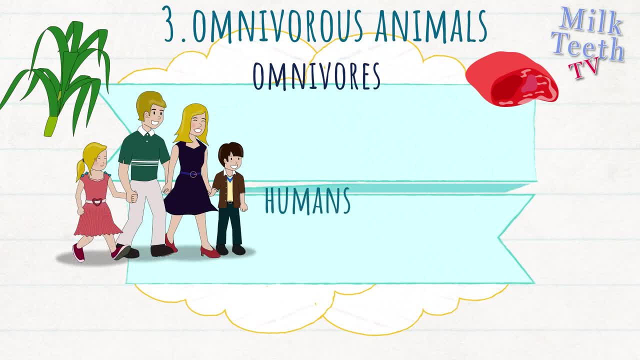 The most important mammal, that is, human beings, eat both plants as well as other animals as a source of their food. The animals are called omnivores, and omnivores are animals that live on lake existence. Theseautocles living in the Ș 지�cholyож heißt hay.